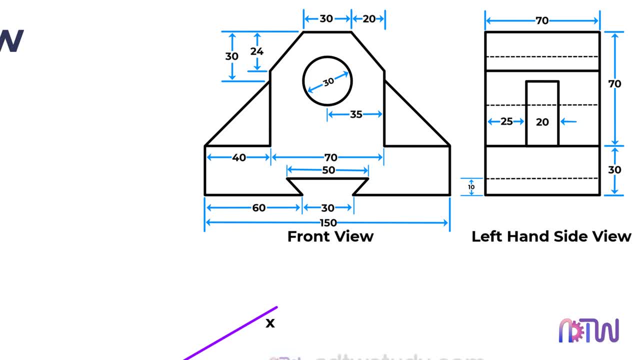 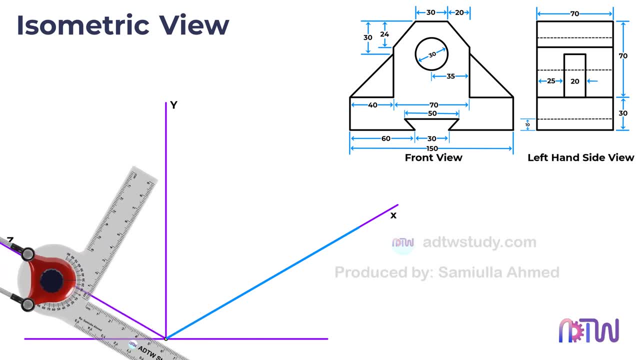 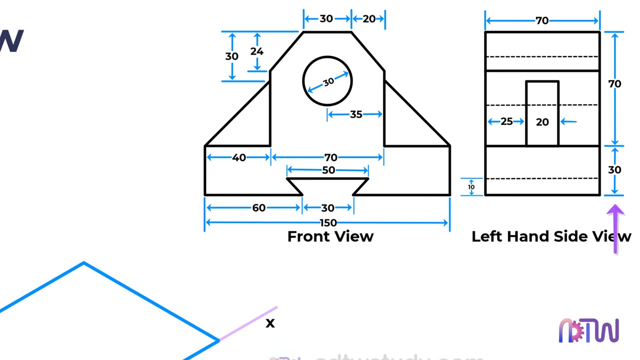 given as 70 mm. Using a drafter, proceed to construct the outline for the base as instructed. Next, in the left-hand side view of the object, we observe that the thickness of the base is 30 mm. To account for this, increase the thickness of the base by 30 mm by drawing vertical lines. 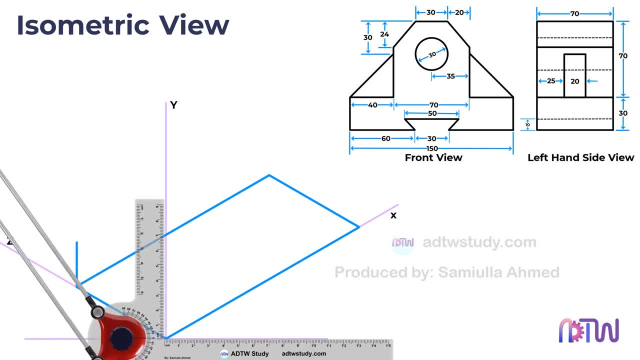 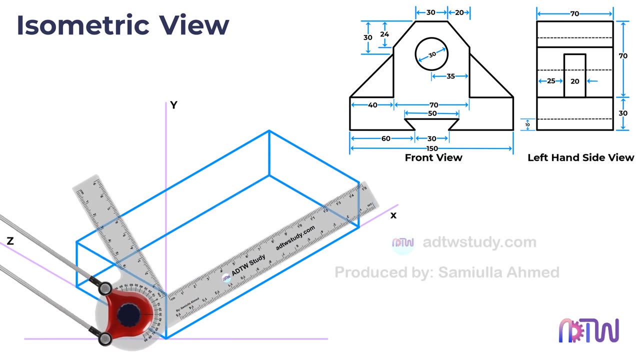 from each corner point of the outline. Finally, join the endpoints of the vertical lines. to complete the base, Draw a line to be defined in theta by 19 mm only. Following the previous steps, we now proceed to draw the inner slot on the base. 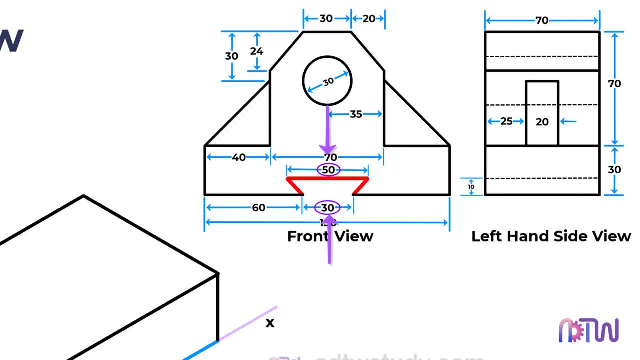 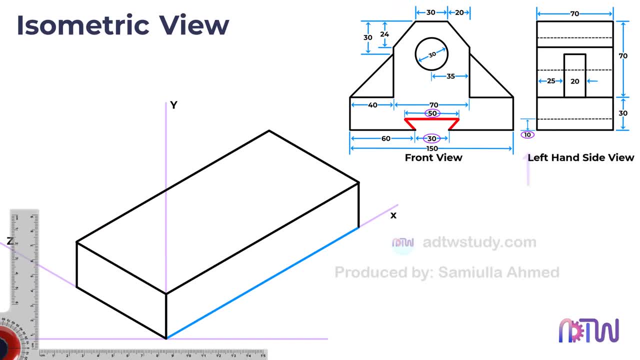 The top width of the base measures 50 mm, while the bottom width is 30 mm. Additionally, the height of the slot is 10 mm. To construct the slot, begin by drawing a line parallel to the x-axis at a height of 10 mm from. 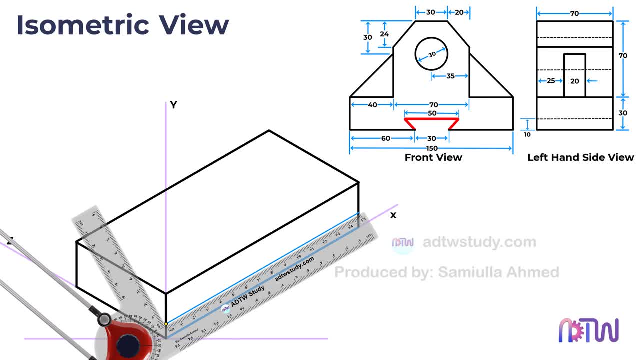 the origin. Draw a line to be defined at a height of 19 mm from the origin. Then mark the mid-point of the vertex of the x-axis. Next, draw the center line of the vertical line of the theoretical elements. This time we will draw a line direct from the què-x axis. 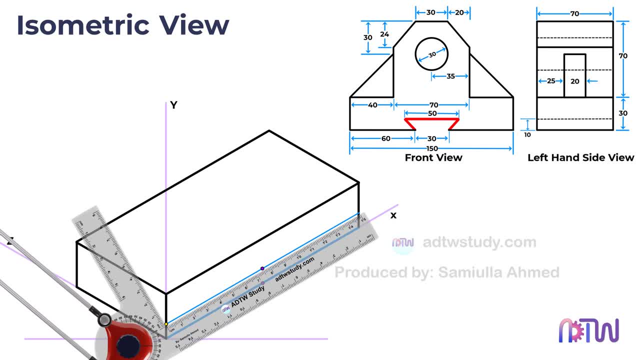 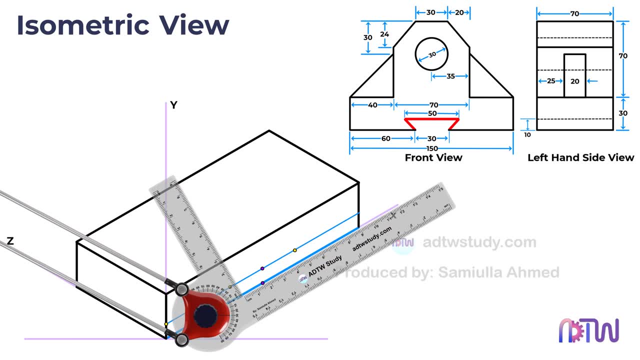 this line From the midpoint. mark points that are 25 millimeters away on both sides. Additionally, mark points that are 15 millimeters away on either side from this midpoint. Finally, connect these marked points to construct the slot. Make sure to include all the required details within the slot. 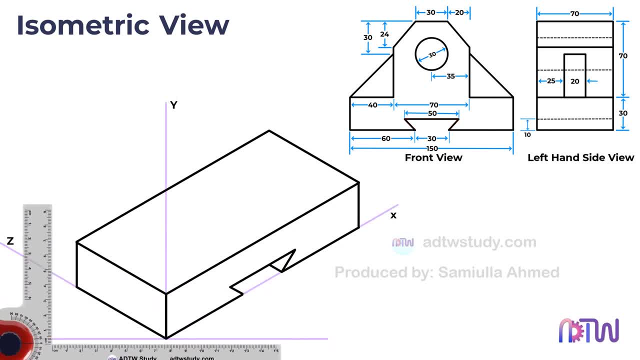 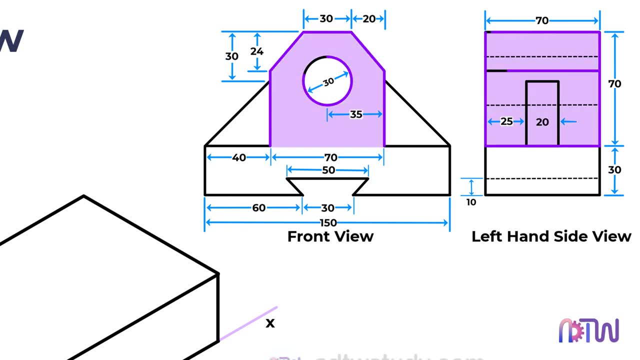 This marks the completion of the base of the object. Now let's move on to constructing the top portion, which consists of two parts: the center portion and the two side portions. The center portion has a width and height of 70 millimeters and it is positioned exactly. 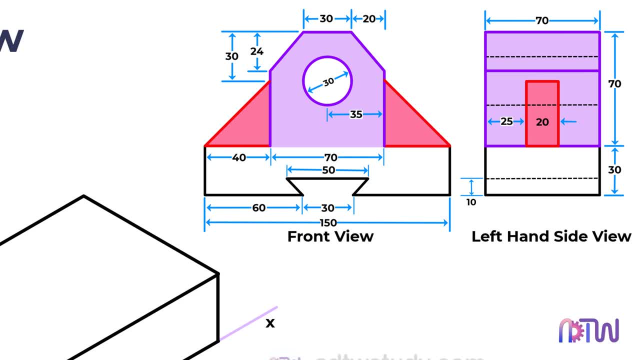 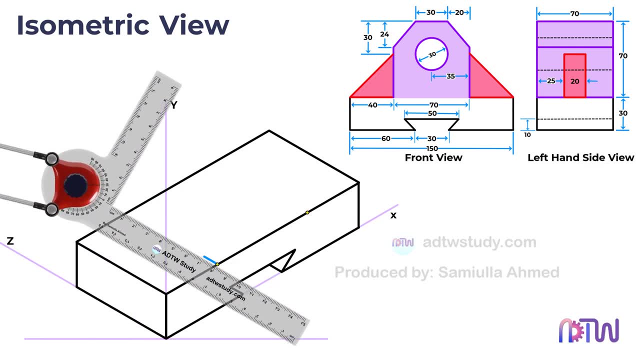 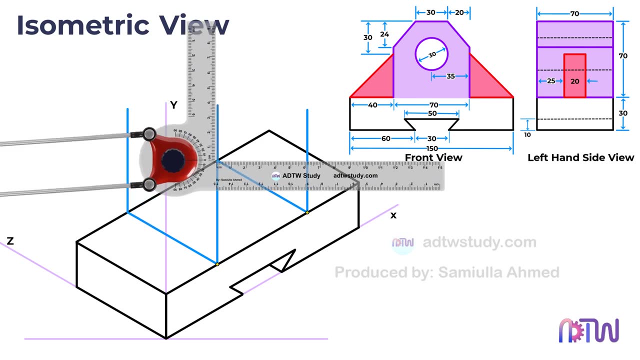 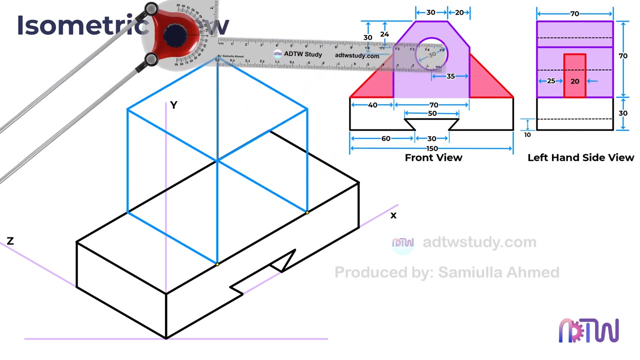 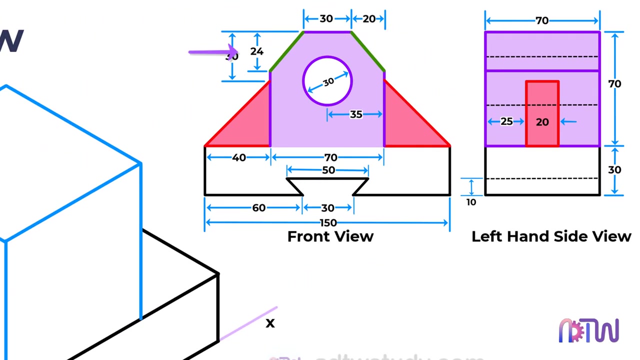 in the center of the base. We will begin by constructing the outline for this center portion. Next, we notice that the two edges of this feature are chamfered. The dimensions of the chamfer are 24 millimeters and 20 millimeters. 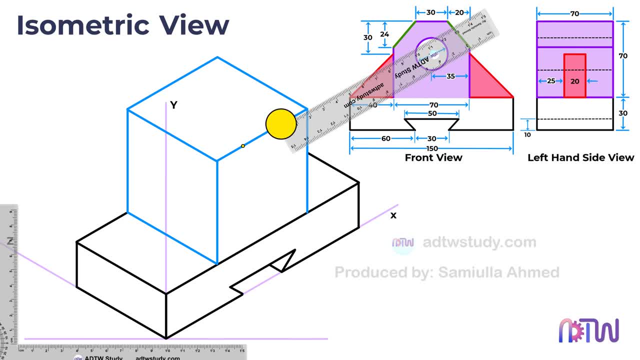 To achieve this, we will mark 20 millimeters on top from both edges and then measure vertically from the top by 24 millimeters on these edges. Afterwards we will draw parallel lines to the z-axis from these points to complete the chamfers. 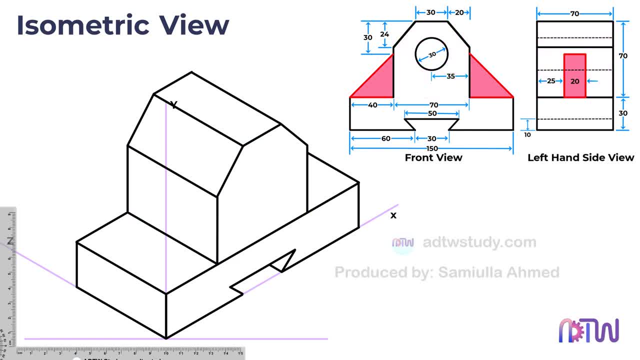 Following the construction of the center portion with chamfers, we now proceed to draw the two side features. Please note that only the left-hand side feature will be visible in the left-hand side view of the object. In the left-hand side view, we can observe that the incline portion has a thickness of 20 millimeters. 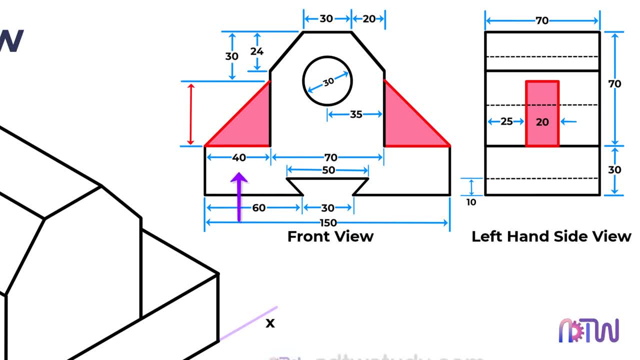 and a width of 40 millimeters. To determine the height of this feature, we subtract 30 millimeters from the 70 millimeters height of the center portion, as shown in the front view. With the required dimensions in hand, let's begin the construction process. Start by marking the center. 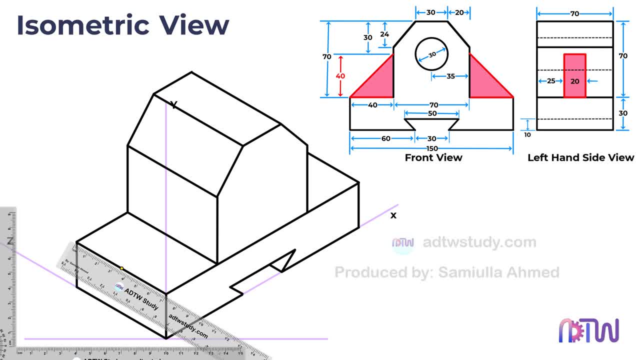 point on the side of the baseline. After marking the center point on the side of the baseline, proceed to mark points at a distance of 10 millimeters on either side. Then mark a point at a height of 40 millimeters from the base and draw a line parallel to the z-axis. 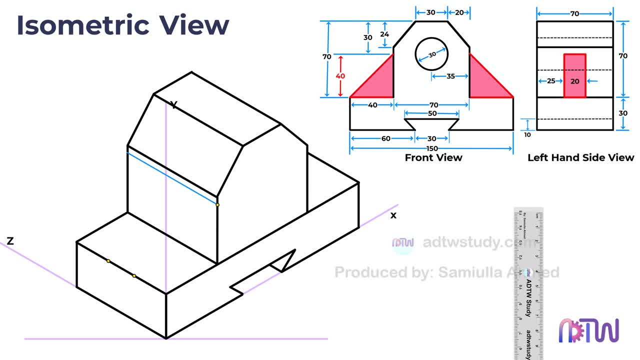 Similarly, mark the center point on this line and mark points at a distance of 10 millimeters on either side of this center point. Finally, connect these points to complete the incline portion. Make sure to add all the necessary details to complete the construction. 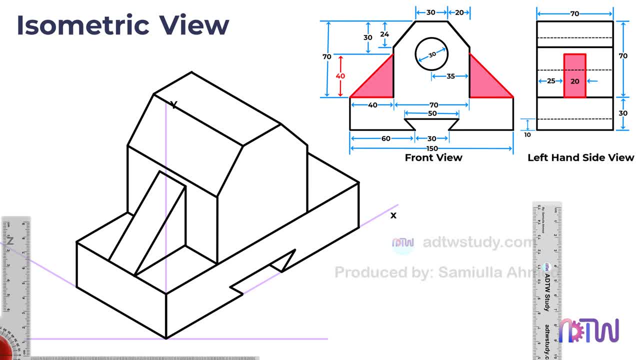 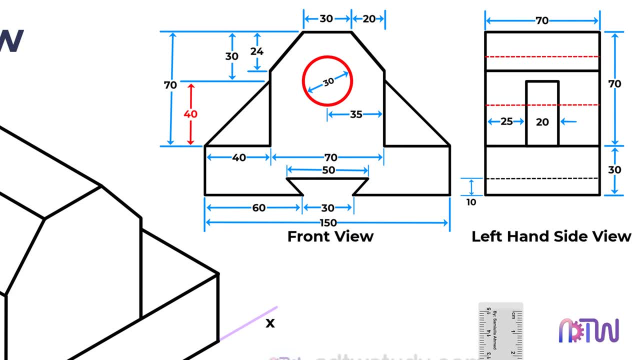 With this step we have successfully constructed the side portion of the object. To draw the 30 millimeters diameter hole on the center portion of the object, we first need to locate its center position. From our observation we can determine that the center of the hole is exactly in the middle and 30 milimeters. 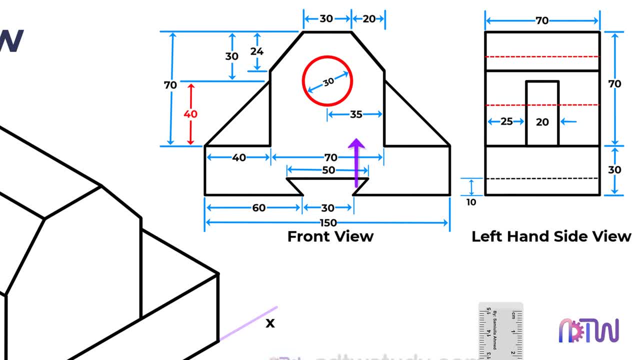 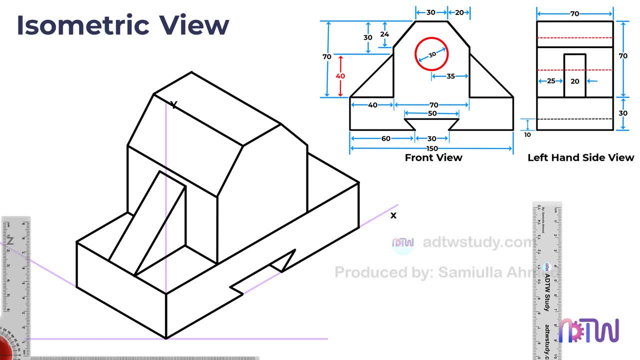 выс saúde checkский получилось. millimeters below from the top of the center portion. To locate the center, draw vertical and horizontal lines. The vertical line should be 35 millimeters away from the side and the horizontal line should be 30 millimeters below from the top. The intersection of these lines. 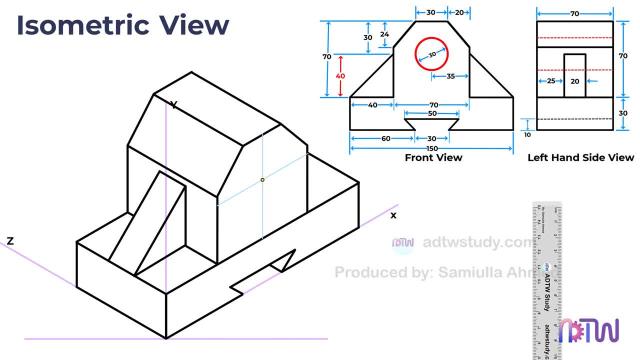 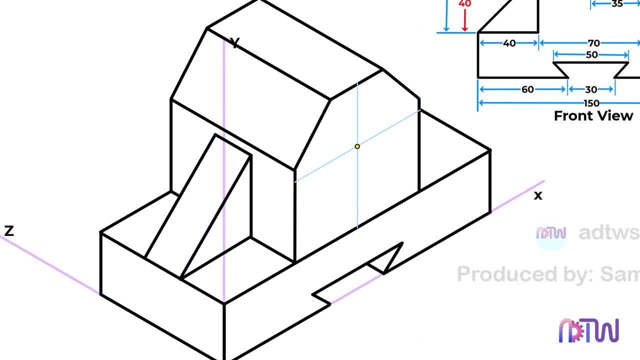 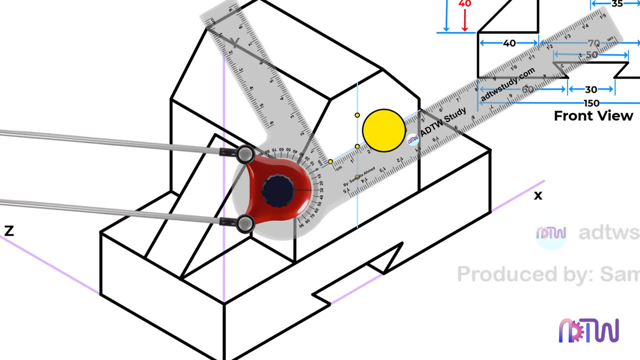 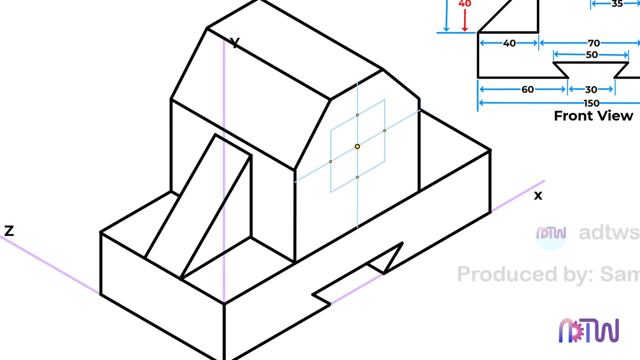 will represent the center point of the circle. Since the diameter of the circle is 30 millimeters, we will construct a square with sides measuring 30 millimeters at this center point. Construct the square as shown. Following the construction of the square, the next step is to draw the diagonals by: 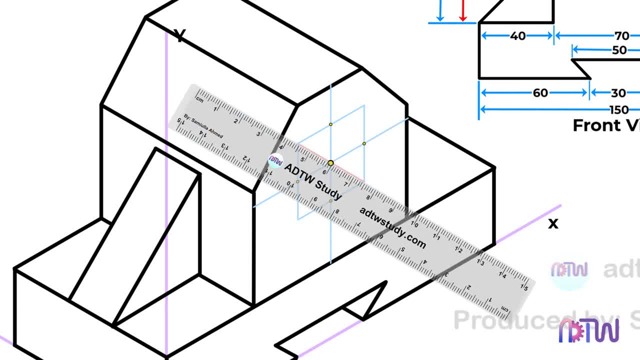 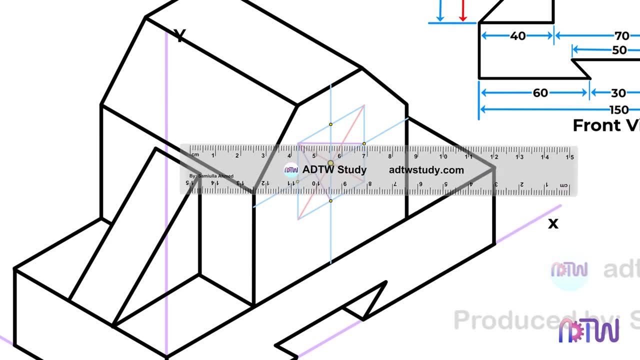 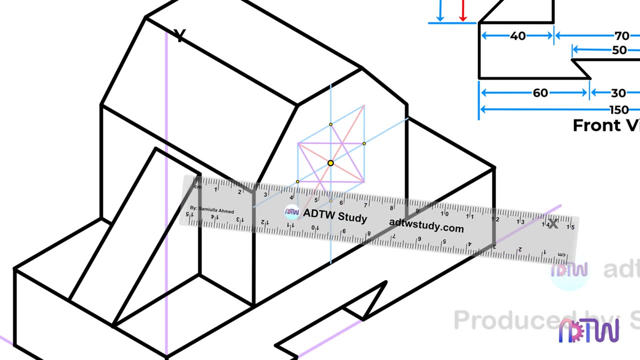 joining the opposite endpoints of the square. This will create an X-shaped pattern within the square. Next, connect one of the diagonal endpoints with the adjacent endpoint. Similarly, connect the other diagonal endpoint with its adjacent endpoint. These lines will intersect with the diagonals and form four points, Using: 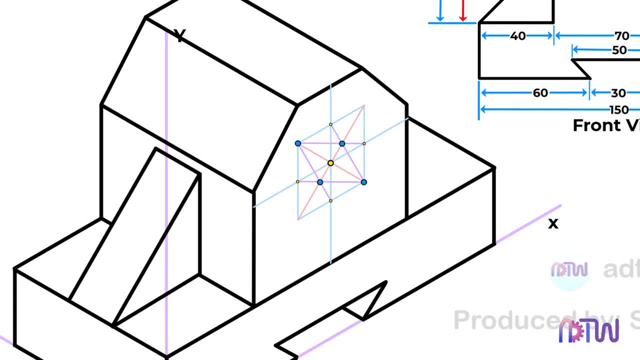 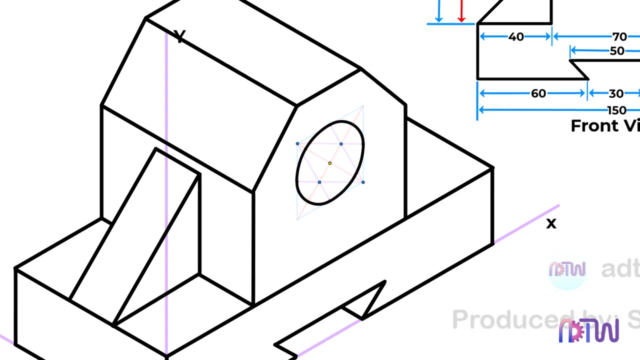 these four points as centers, draw arcs as shown in the diagram. These arcs will form the curved edges of the circle in the isometric view. Additionally, using these two points as centers, draw arcs to complete the circular shape of the whole. By following these steps, we successfully draw the circle in the isometric view of the. 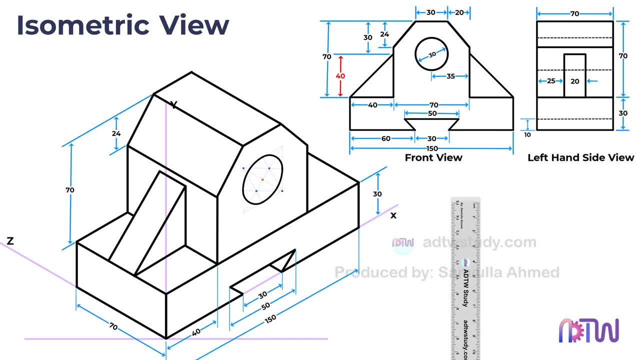 object do the dimensioning of the figure. This is the final required figure. I hope this tutorial helped to understand how to construct the isometric view of an object from its orthographic projections. If you found this video useful, please give it a thumbs up by clicking on. 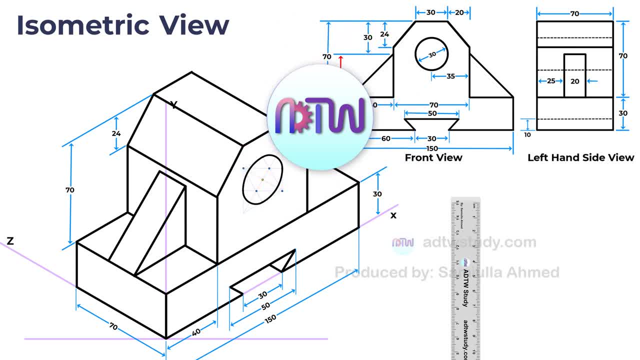 the like button And if you're new to my channel, ADTW study, make sure to hit the subscribe button to stay updated with all my latest videos.